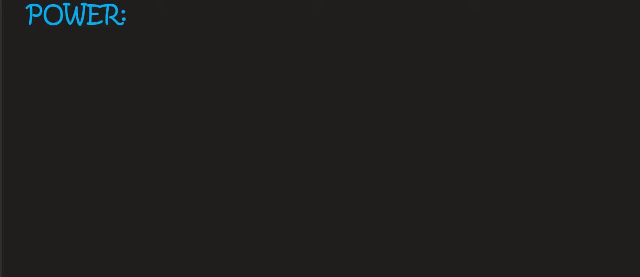 Hello guys. so if you managed to get through the previous section on mechanical energy and work easily, then power is going to be an absolute breeze. The definition of power is the following: Power is all about how fast the energy or work is done. Now, that's obviously not the technical. 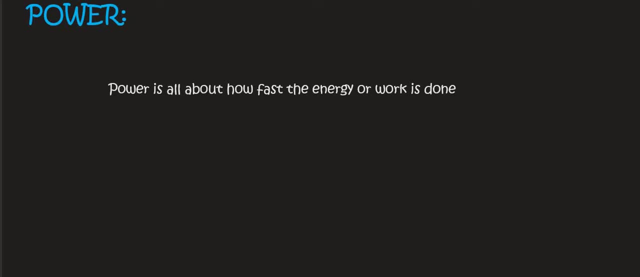 definition. that's just Kevin's definition. So think about this. let's say you've got a water pump that is busy pumping water into a swimming. Now let's say this is pump A and let's say it fills 10,000 liters of water and it takes 24 hours to do that. Then let's say: your neighbor. 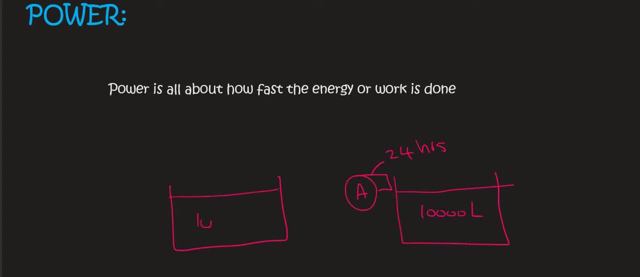 also needs to fill up his pool, his or her pool, and that's a 10,000 liter pool. They're using a different pump, which I'll call pump B, and their pump takes 16 hours. Both pools are doing the same amount of energy or work. they're both filling 10,000 liters. However, your neighbor's pump, which 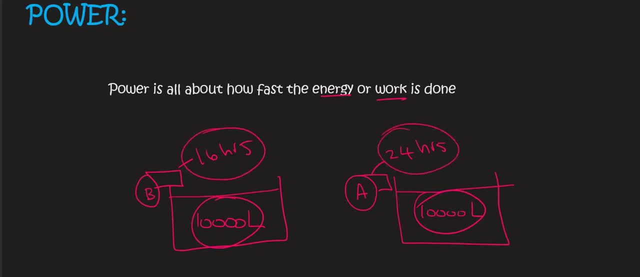 is, pump B takes 16 hours, whereas your pump takes 24 hours. We would therefore say that your neighbor's pump is more powerful because it can do the energy or the work much faster. So in formula terms, power is equal to the following: So power is equal to the: 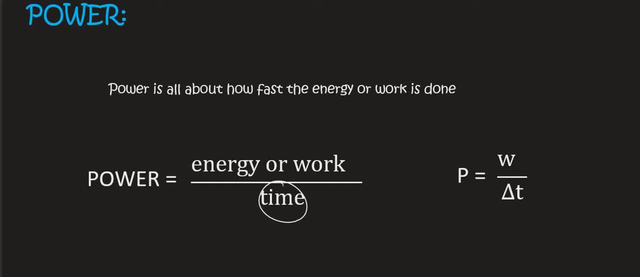 energy or work divided by the time. In formula terms- and you do get this on your formula sheet- it's equal to W, which stands for work. but remember that's the same as energy divided by the change in time. There is another formula for power, but I'll have to show you that in a later lesson, when. 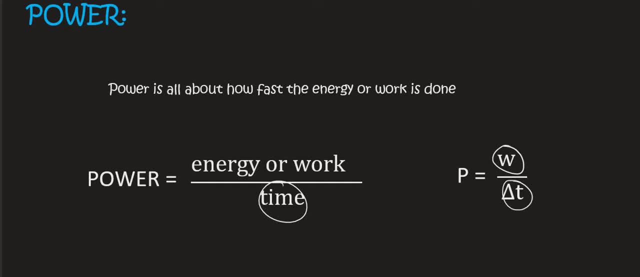 I'm going to show you how to do that. For now we just think of power as the amount of work or energy divided by time. So it's very simple, because if you know how to work out the energy- which we'll typically use this formula over here- then you've got the time typically, and then you can work out. 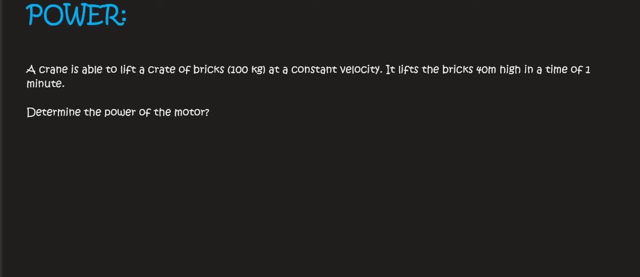 the power. So let's practice a bit. So here we have a question where we have a crane that is able to lift a crate of bricks which have a mass of 100 kilograms at a constant velocity. It lifts the bricks 40 meters high in a time of one minute. Determine the power of the crane. So we have a. 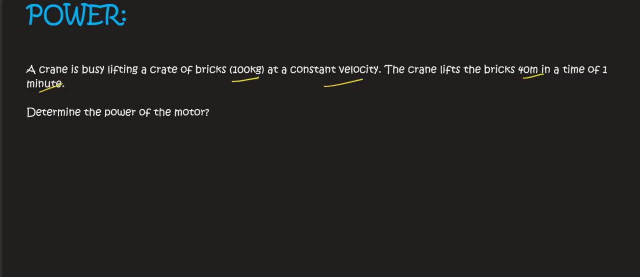 motor. So we know that power is equal to and so if we could work out the work, then we can work out the power. So work is equal to the force times by the displacement times by the cos of theta. So if we have a pile of bricks, we've got this motor that's trying to lift them upwards and 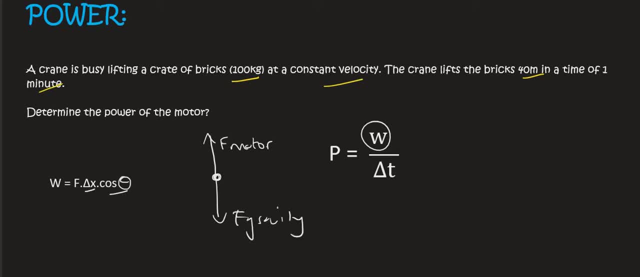 then obviously there's gravity. Now, because we are moving at a constant velocity, it means that those two forces must be balanced, and so the motor will be the same as the force of gravity, which is just the mass. So if we have a pile of bricks, we've got this motor that's trying to lift them. 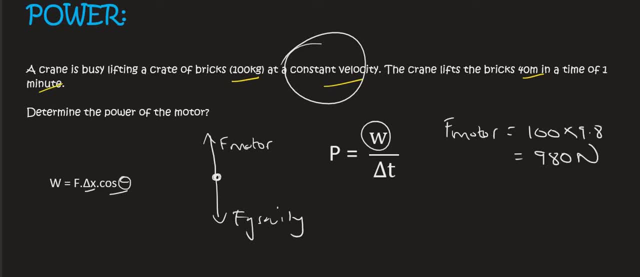 by the mass times by 9.8, and that's going to give us 980 newtons. So then the work of the motor will be 980 times by the distance, which is 40 meters. Now the crate is busy moving up and the motor is. 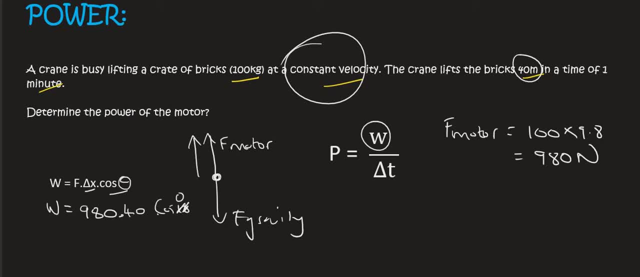 moving or working upwards, and so that's cos not 180, cos 0, and so then 980 multiplied by 40 is going to give a work of 39,200 joules. So then we can say: power is equal to the force times by the. 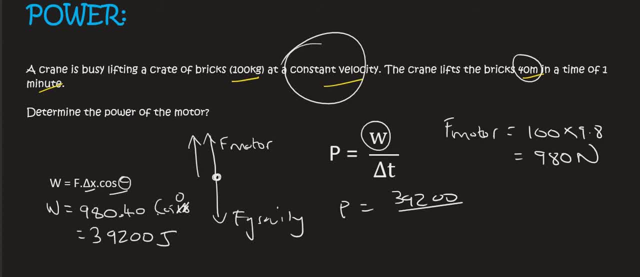 time. but now time must be in seconds, and so if you do that, you end up with 653.33.. Now, power is measured in watts. Now, I'm not asking you what it's measured, I'm telling you it's measured in watts. So that's just a silly little joke. it always catches my students. So power is measured. 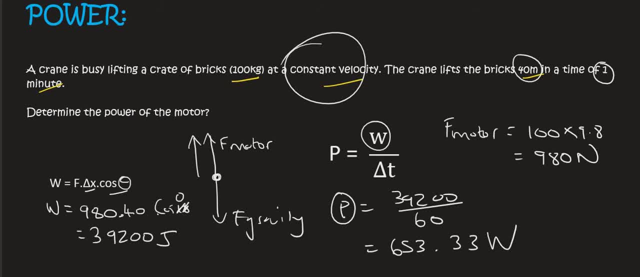 in watts Now, something that's very interesting, and this is where the second definition of power arises, and I see them do this in exams a lot. I could have left out the distance and I could have left out the time, but I would have given you. 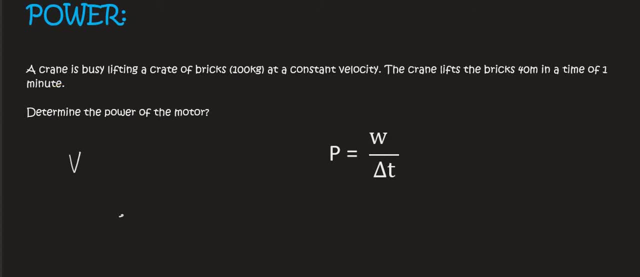 the velocity, because have a look at the following: We know that velocity is equal to the change in the displacement over time. So I have that information, I've got 40 meters and I've got one minute, So I could say that the velocity is equal to 40 over 60, which is going to give you 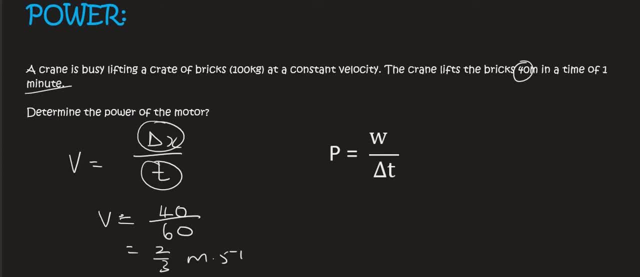 2 over 3 meters per second. That is how fast the bricks are moving. We can say that for sure because it's moving by the time. So I could have left out the distance and I could have left out the velocity. Now what I'm saying is that velocity is moving at a constant velocity. It might have